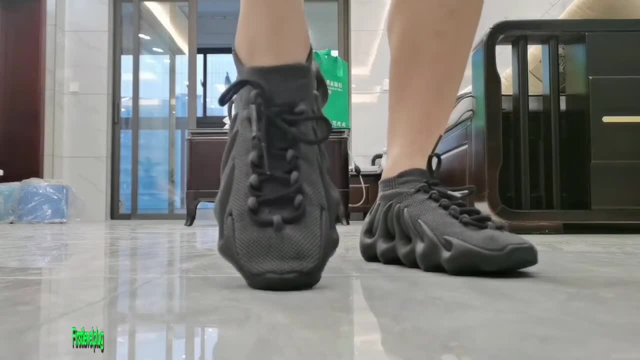 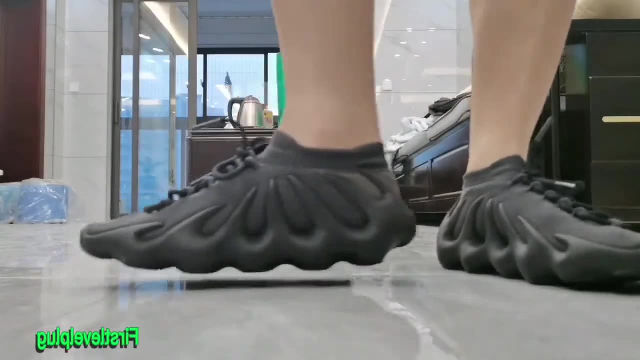 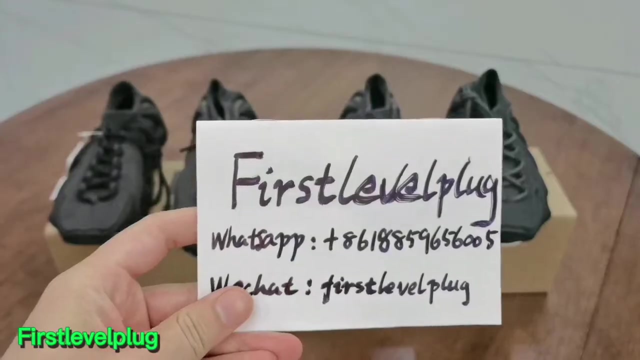 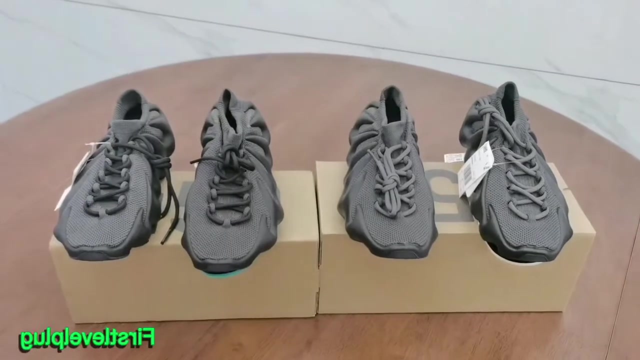 Today we will compare the difference between the two pairs of DC450.. I will compare our gold version to some cheap version so you can know how good quality our gold version is. Our gold version is the same as the retail one. It's 100% the same as the retail one And the triple fake. there are some faults here. 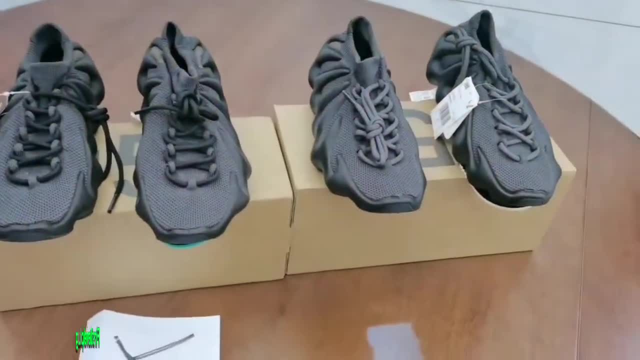 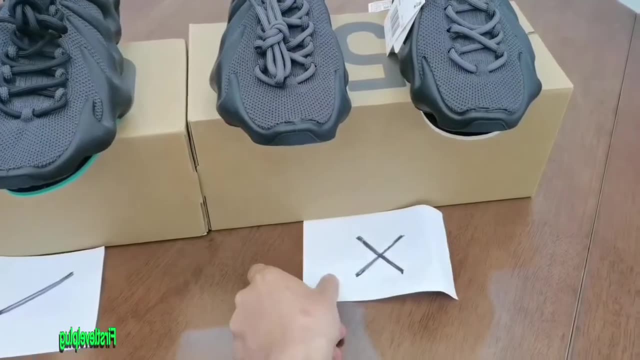 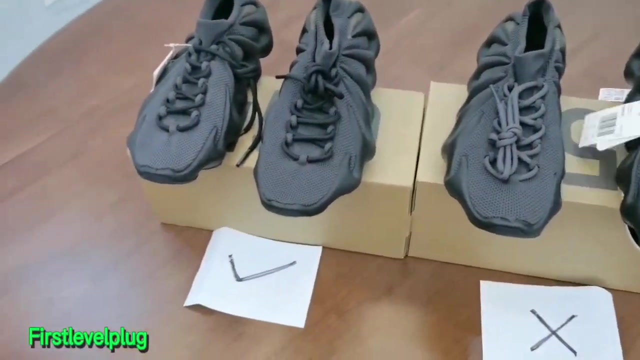 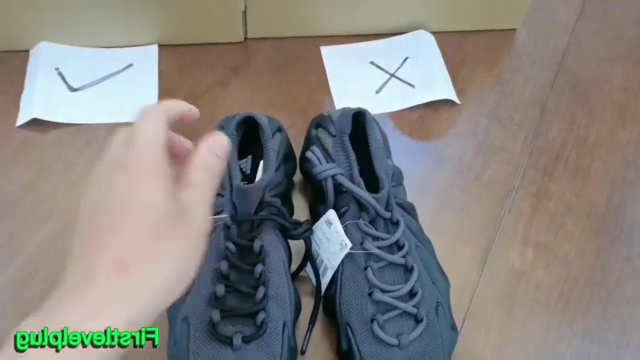 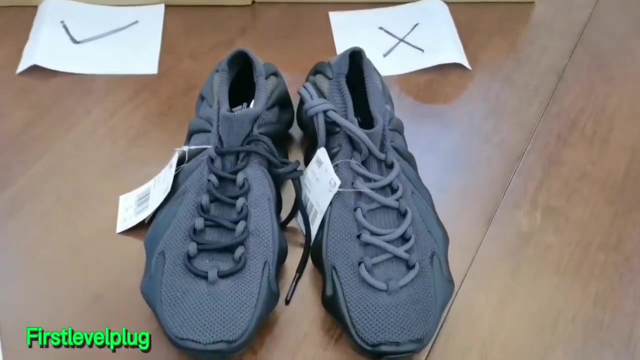 On my left it's the gold version and it's correct, And on my right it's the cheaper version. It's incorrect. What's the difference? Let's move on to the details And first check the shoelace: Absolutely the gold version. the shoelaces is dark. 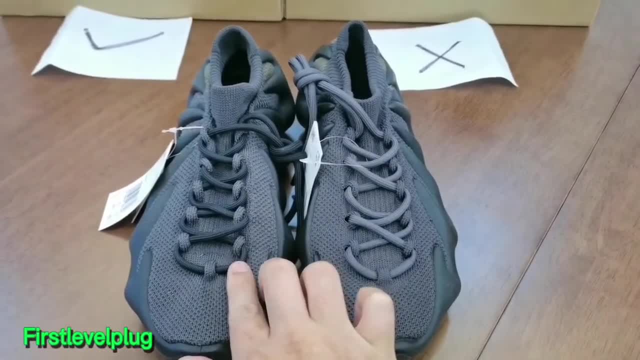 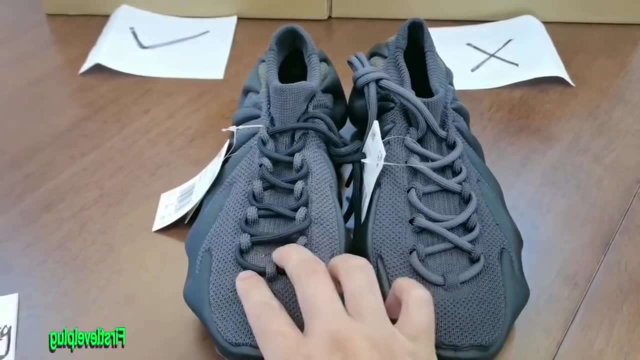 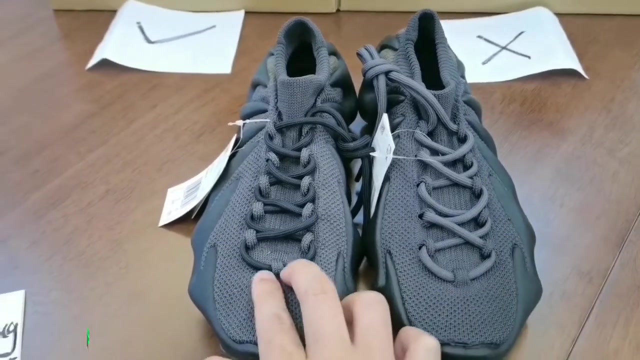 It's dark And it's the same as the retail one And the cheaper fake. its shoelaces is gray. It's incorrect. This is the difference of the colorway. This is the different colorway you can choose from. If you want to find the difference, you have to pay more or get it before. see the gold version. 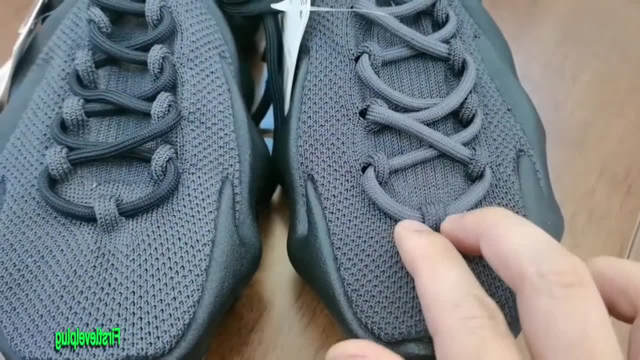 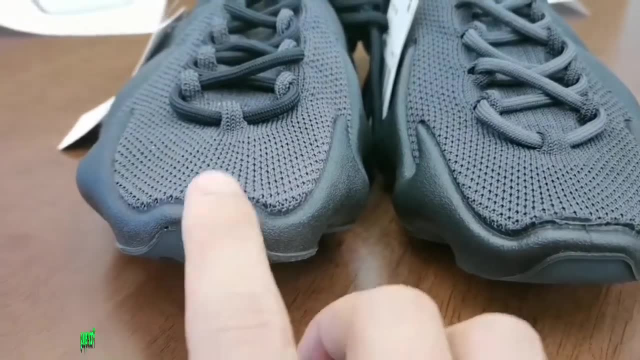 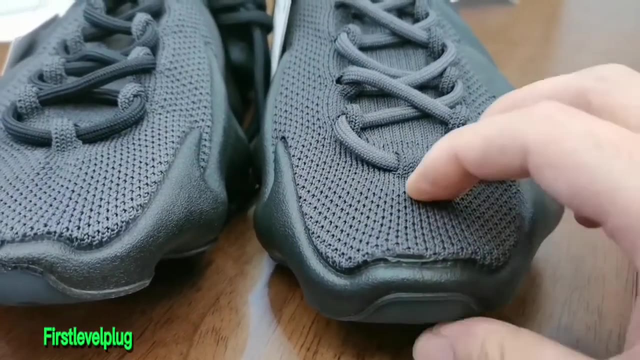 It's only about 80% of the gold version you can buy for the dollar. It's similar to the original quality. To get the different color of the gold version, you are going to buy the Dohyond type or or dual colorway version if you already have four colorways. 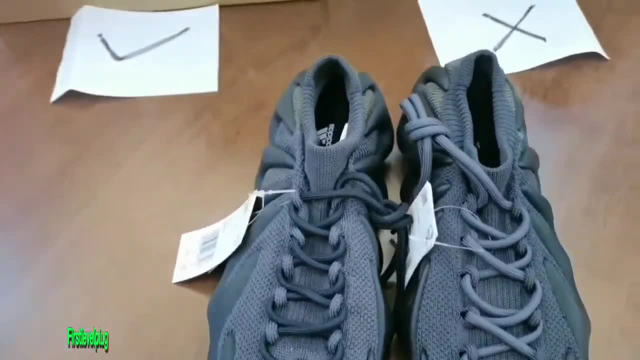 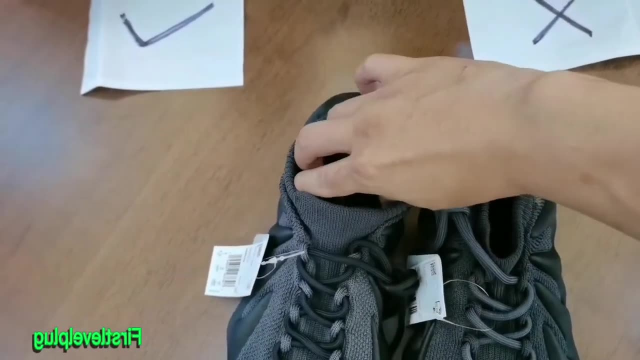 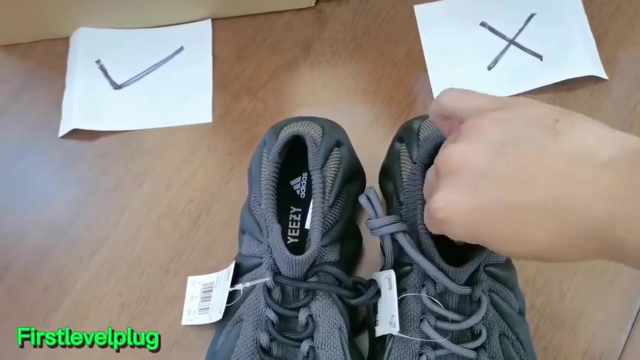 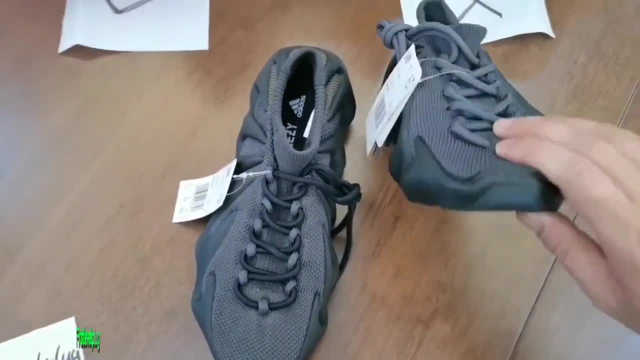 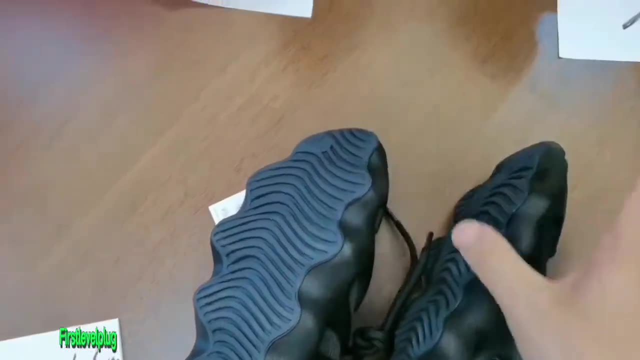 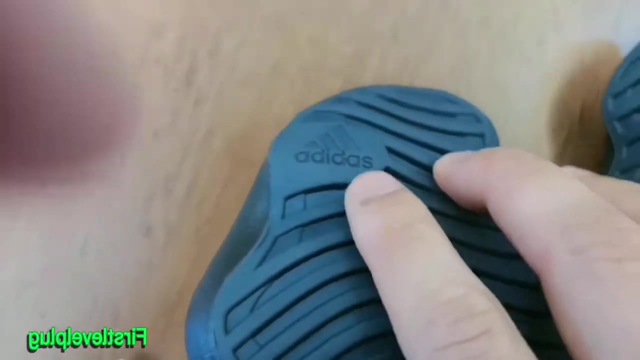 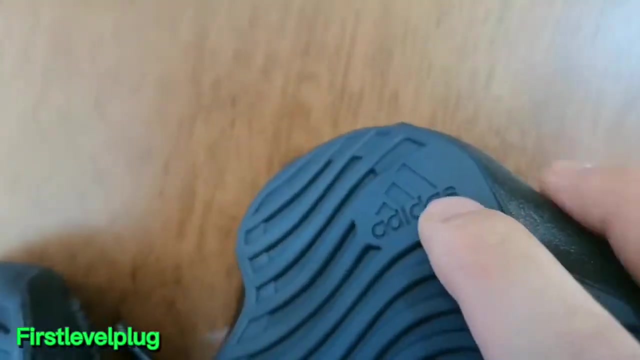 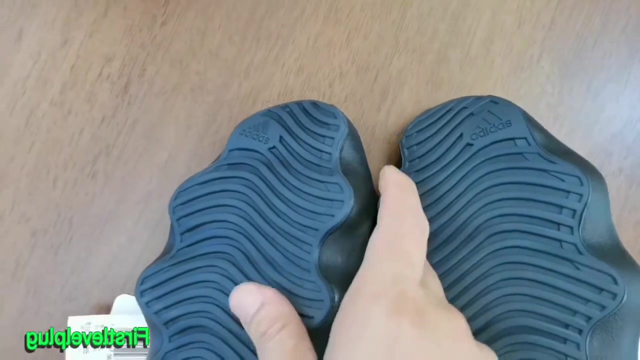 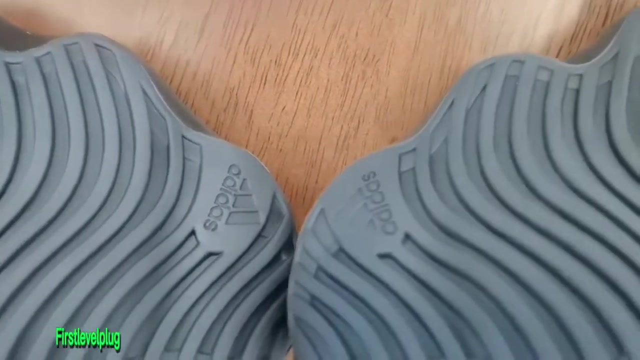 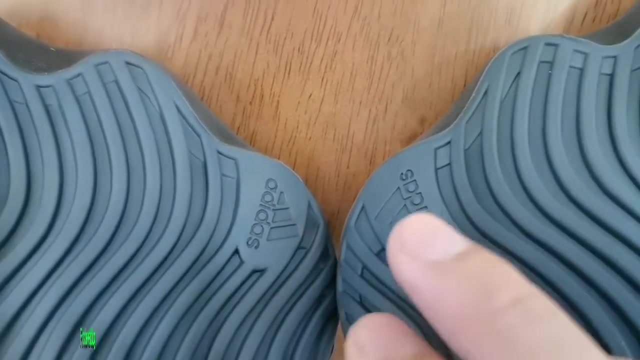 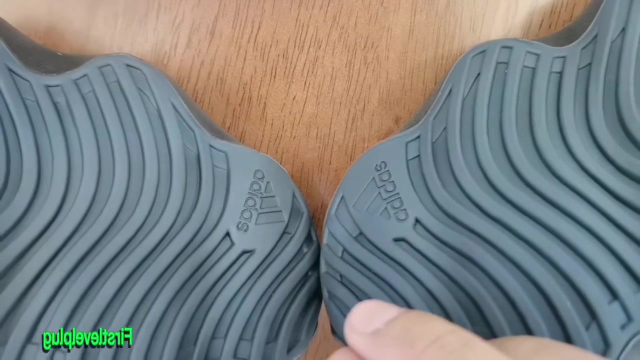 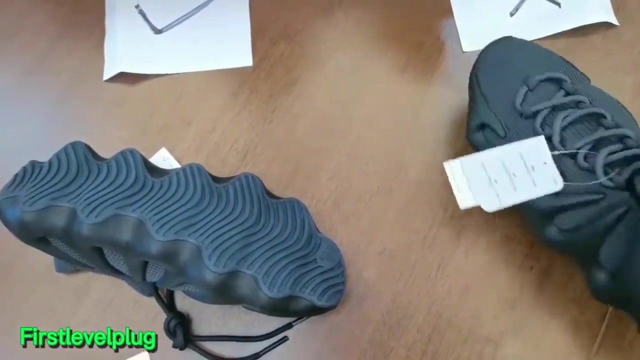 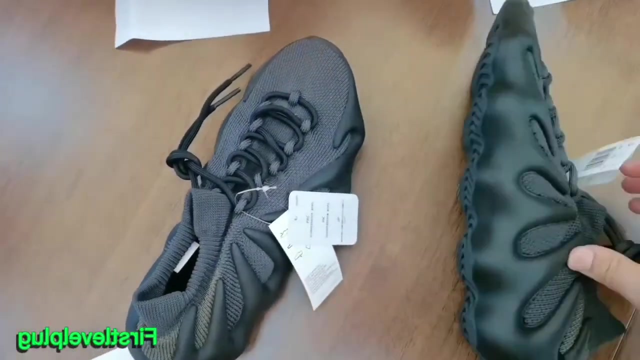 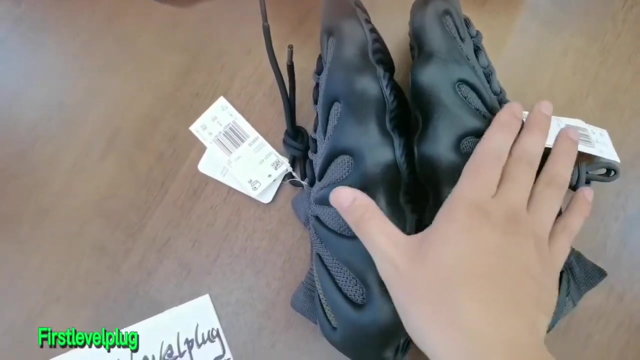 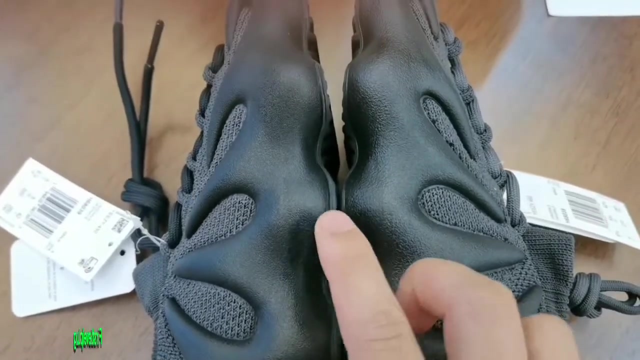 cheaper version incorrect, then let's move on to also check a local Adidas. our got a version. the local it's right and the triple fake tap face is the wrong and you can see this to pair them. does our material got a version? this part is low and 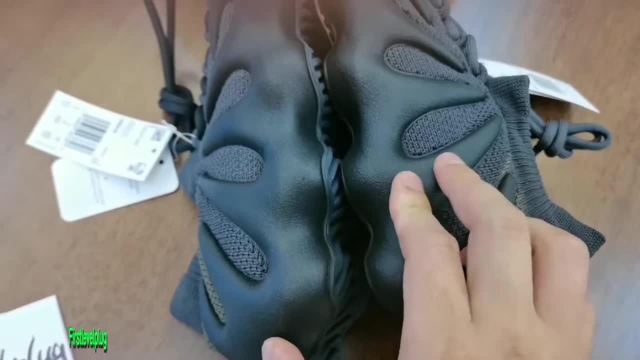 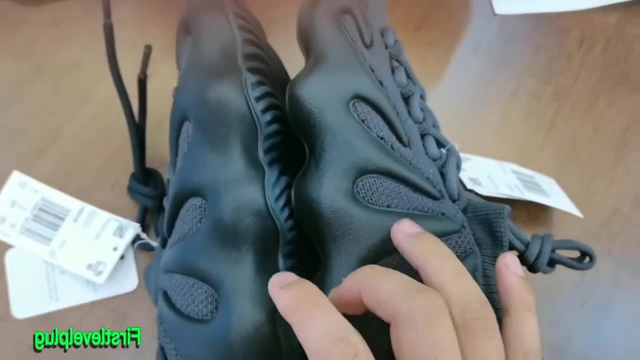 sensor retail one, but the version is not. the version is not the real one, but the version is not the real one. but the dual fake this part, it's delicate. and if dual fake this part, it's delicate. and if dual fake this part, it's delicate and if we apply them, you will find- look at a: 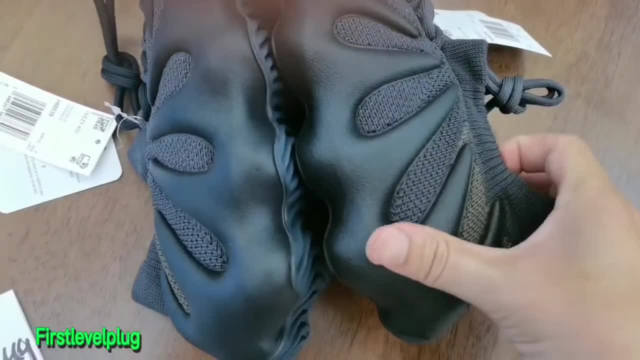 we apply them, you will find. look at a. we apply them, you will find. look at a version: it's soft and elastic, but the version it's soft and elastic. but the version it's soft and elastic, but the triple fake it's hard and elastic. and triple fake it's hard and elastic. and 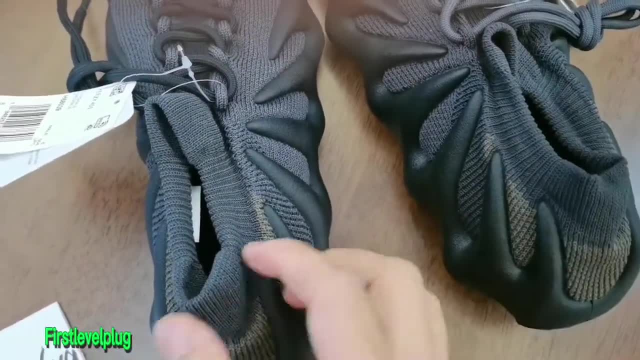 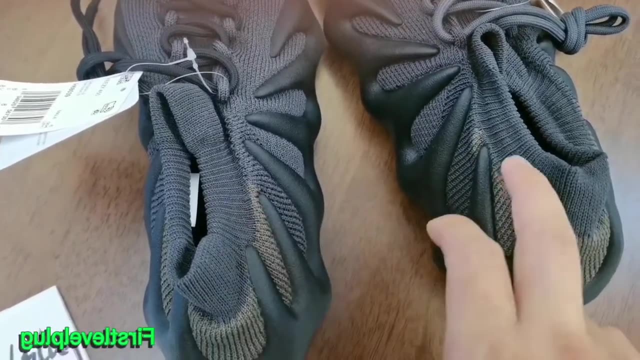 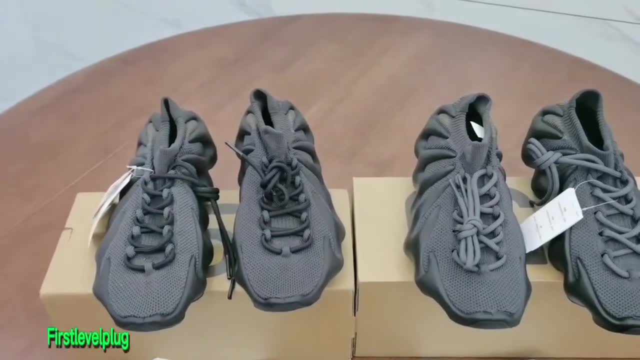 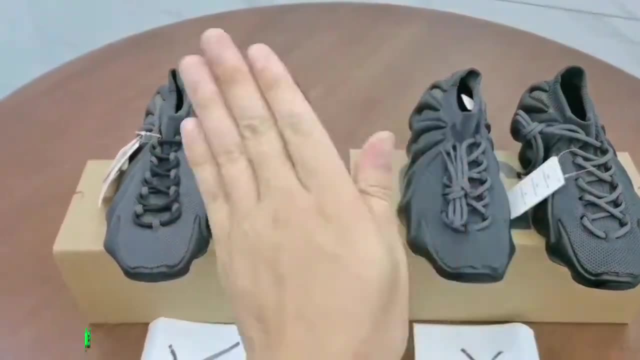 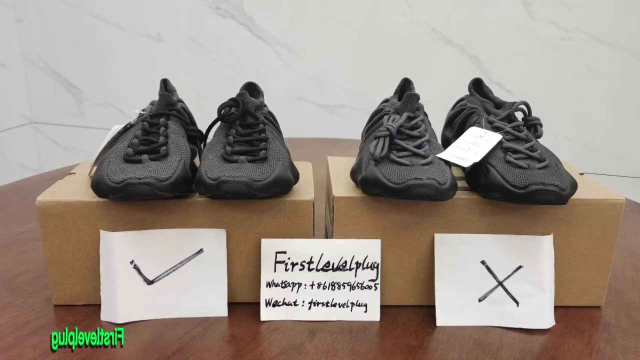 It's incorrect. OK, above of these are the main difference between the two pairs of shoes. I hope it will help you, And the next step is to show you the pair of our God version. Thank you for watching this video. Hope this video can help you.